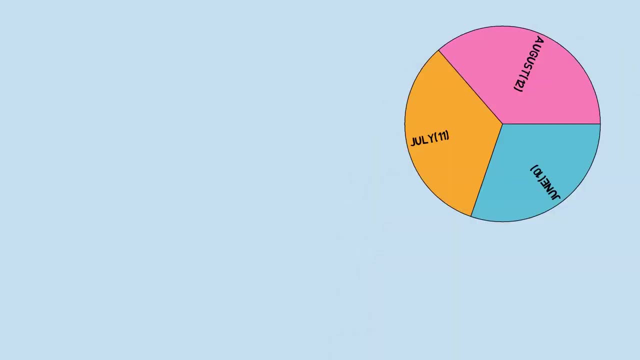 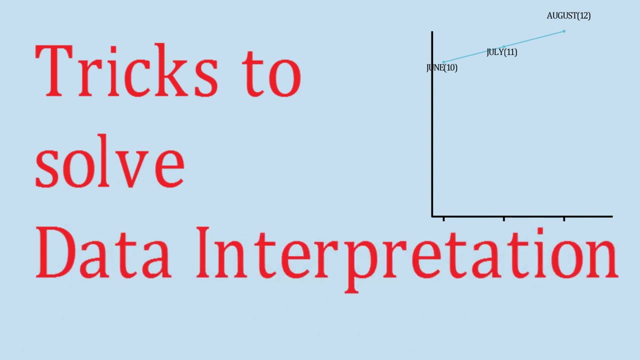 Data, as we know, is a collection of useful information and it can be represented in various ways, like in the form of a pie chart, in the form of a bar graph or in the form of a simple line graph. So what is the actual importance of the representation of this data? It is actually the analysis and interpretation of data. 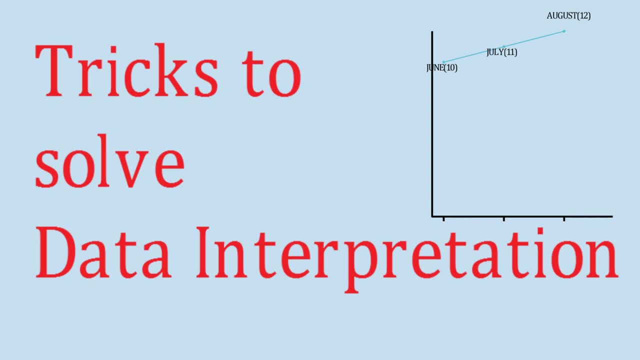 The organizations use this interpretation of data in order to carry out their business in a more effective manner, And that's why it is very essential to understand this concept. OK, if you want to go into a very good company or an organization, you must understand this. 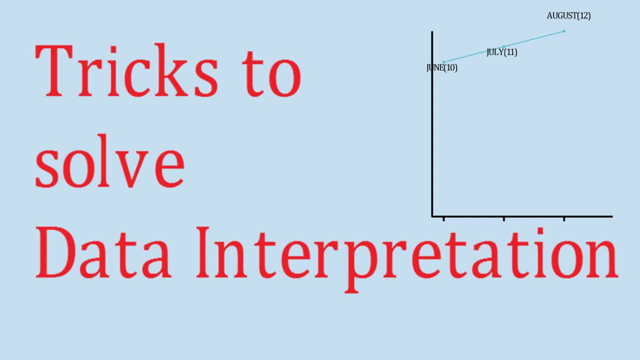 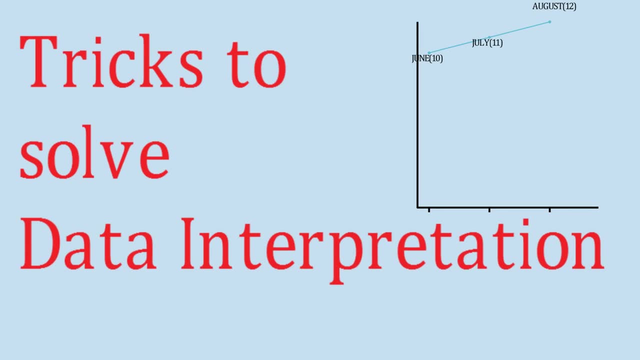 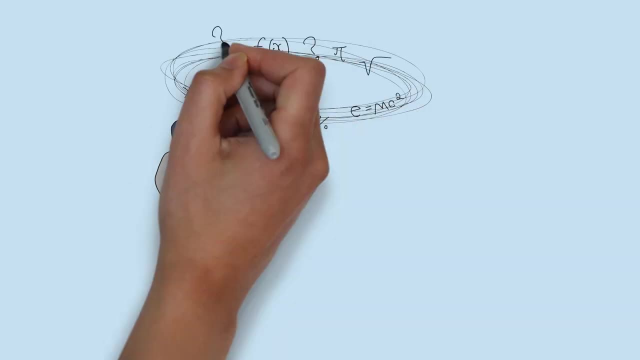 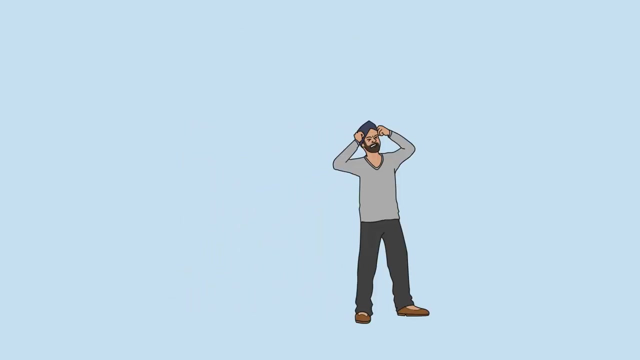 And that is why companies prefer these type of questions in the examination. So when we solve these type of questions, we come across very lengthy calculations. We literally pull our hair when we solve these type of questions. We think of all these concepts of the world in order to solve these questions and end up getting frustrated. 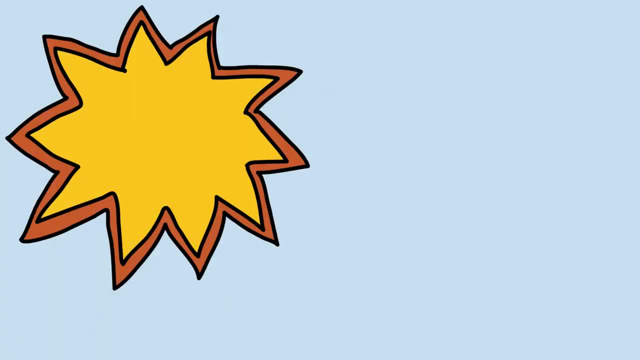 So our focus is to build up these concepts using shortcuts and tricks. OK, the main golden statement which I am talking about is: don't do it the hard way When it comes to data interpretation. do it in the smart way, or the smartest way. 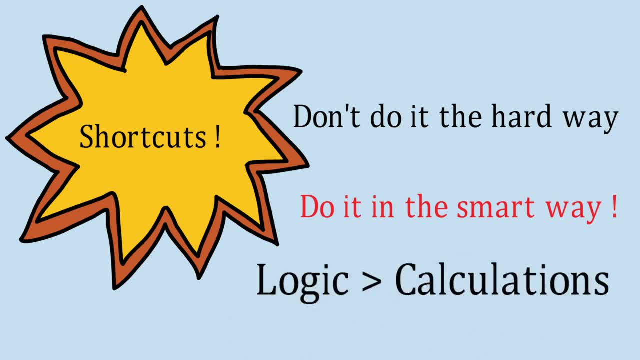 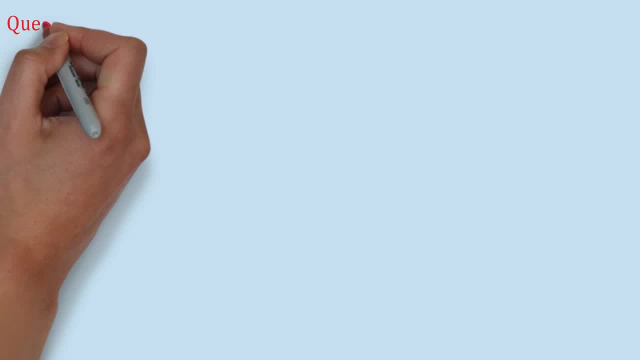 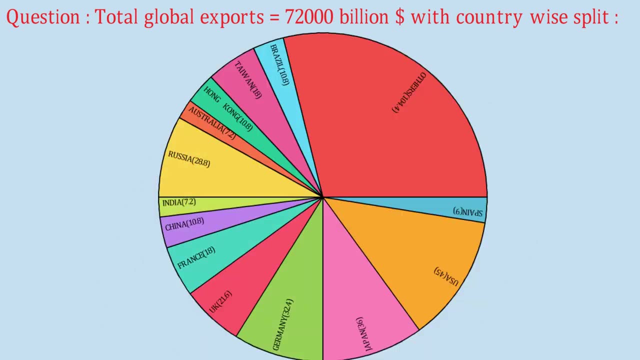 Always remember that logic is greater than calculation. So we will focus more on logic and less on calculations. Let us see the question. The question says that the total global exports are equal to $72,000 billion with country-wise split. So the country-wise share of their exports are represented in the form of a pie chart. 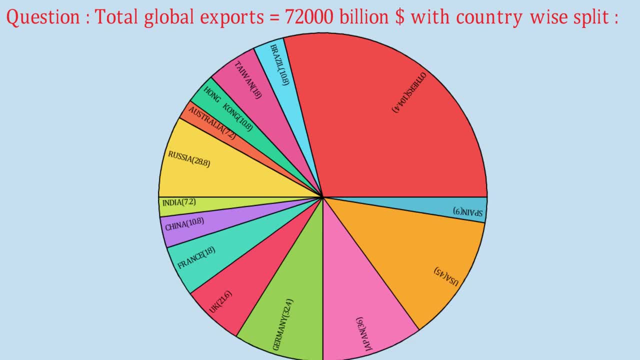 These are the names of the various countries, like Brazil, Taiwan, Hong Kong and all, And in the bracket which is given in the front of each country, like Brazil, 10.8.. So that is a 10.8 degree. We know that the entire angle covered by a circle is 360 degree. 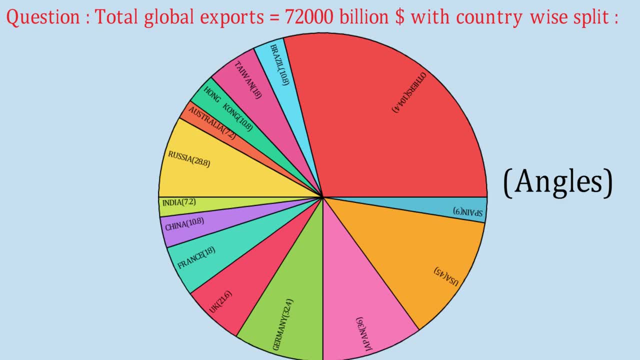 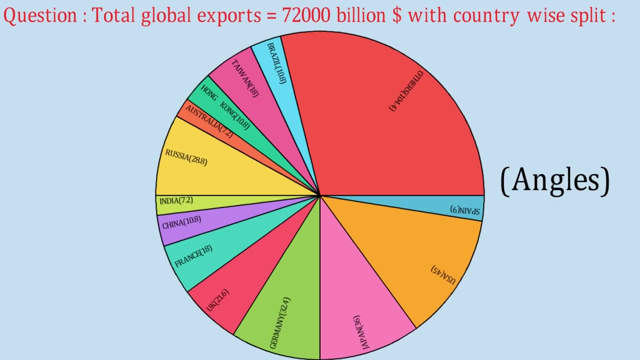 So when we say that Taiwan is having 18 degree, we know that Taiwan is having 18 degree out of 360 degree share. The exports are $72,000 billion. So let us move ahead with the questions based on this data interpretation problem. 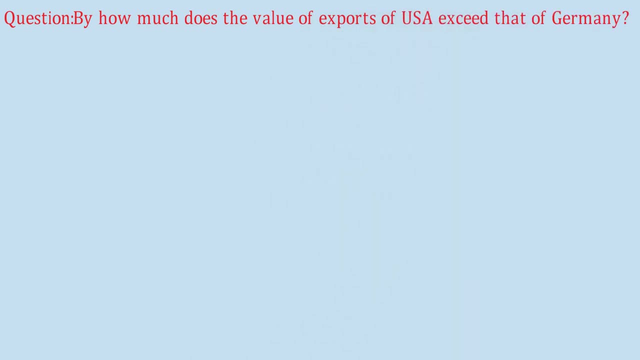 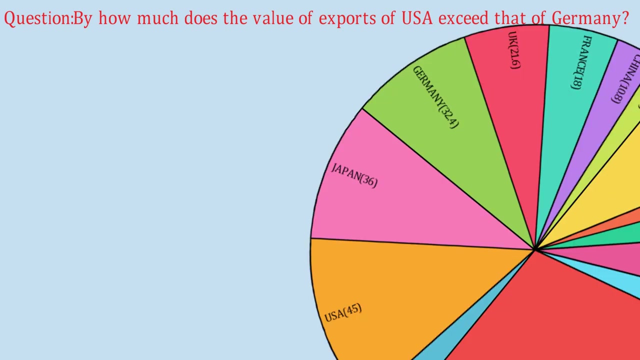 The question is: first question: By how much does the value of exports of USA exceed that of Germany? So when you see the question you must have thought that will come into your mind that let us calculate the exports of USA, Then let us calculate the exports of Germany. 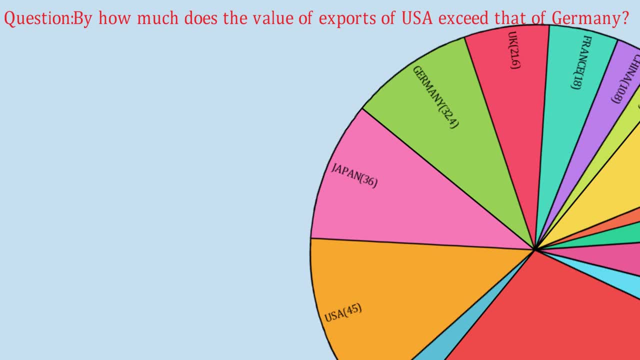 And then we will find a difference in that. But that's not the smart way, That's the hard way. So, when we talk of the smart way, just directly subtract the angle between the two and then carry out the calculation. Okay, Yes, you can directly subtract the angle. 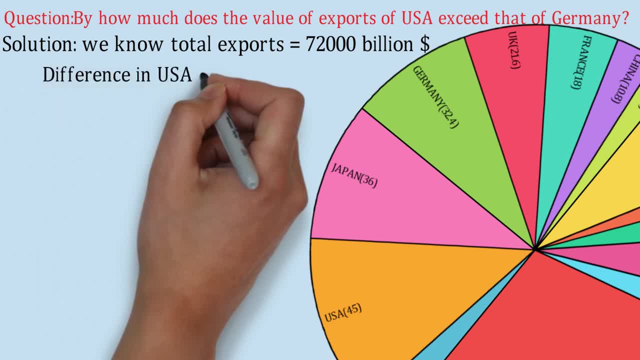 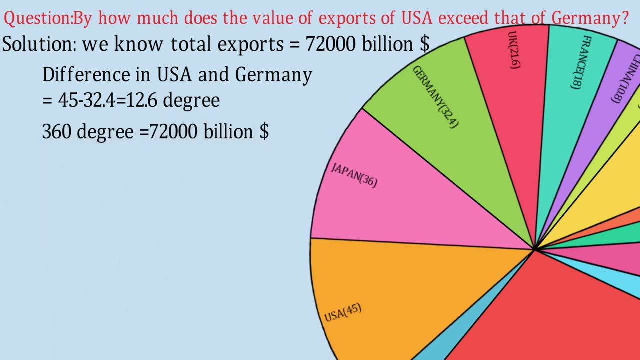 So difference in USA and Germany is 45 minus 32.4 degree, So that is 12.6.. So in the question it is given that the total global exports are 72,000, which means that 360 degree equal to $72,000 billion. 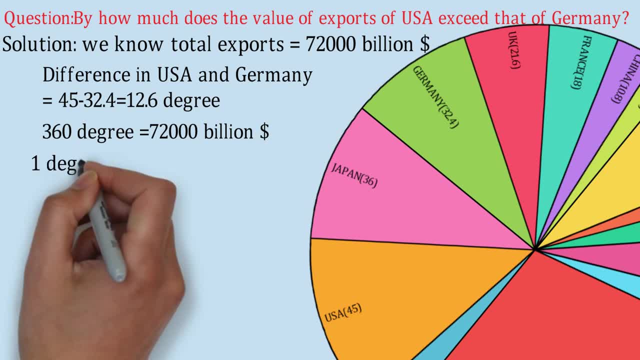 So what does it mean? That one degree is equal to 72,000 by $360 billion. So this means that 12.6 degree equal to this, 12.6 multiplied by 72,000, by $360 billion. So as we solve it, 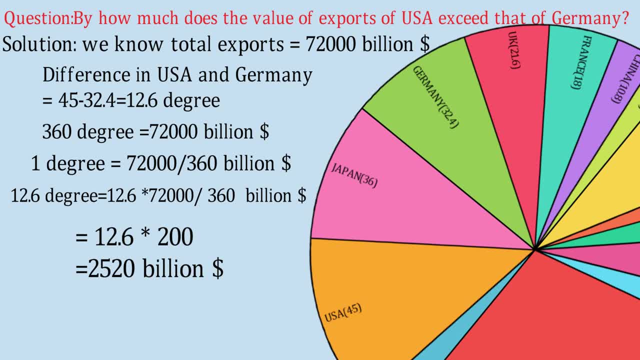 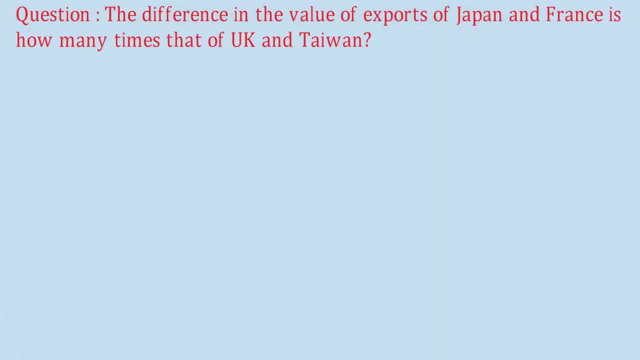 you will get the answer: 2520 billion dollars. So that is how these are little shortcuts, These are little logical things which you must apply in order to solve the data interpretation questions. Next question based on the same problem is: the difference in the value of exports of Japan and France is how many times that of UK and Taiwan? 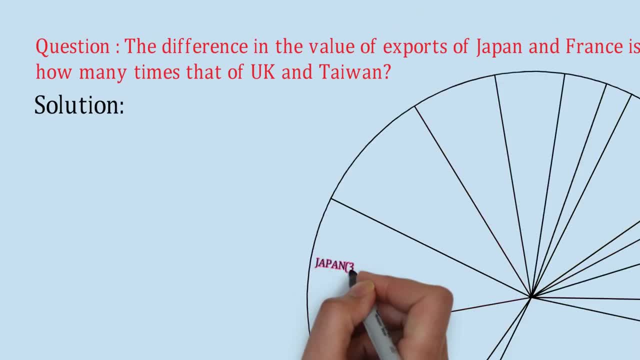 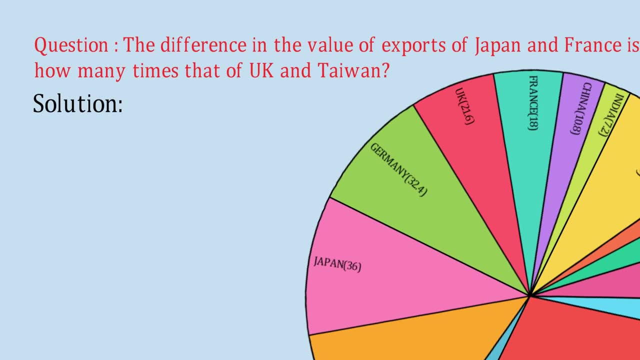 So we need to find the difference in Japan and France, and then you can Taiwan, and then we have to correlate those two differences. So, as we see the question, we need to firstly find out the difference between Japan and France. So, as discussed in the previous, 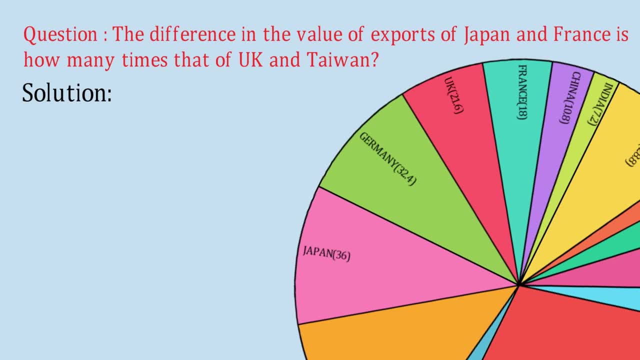 we carry out the difference in the angles of Japan and France. So in the problem Japan is 36 degree and France is 18 degree, So the difference comes out to be 18 degree. Then comes the difference between UK and Taiwan. So the value for UK we can see is 21.6 degree. 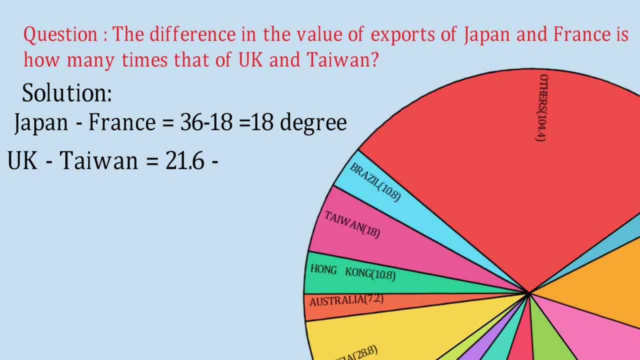 And what is for Taiwan? Let us rotate it. The value for Taiwan is 18 degree, So it is 21.6 minus 18 equal to 18.6.. 18 minus 18 equals to 3.6 degree. So now we have to just calculate how many times. 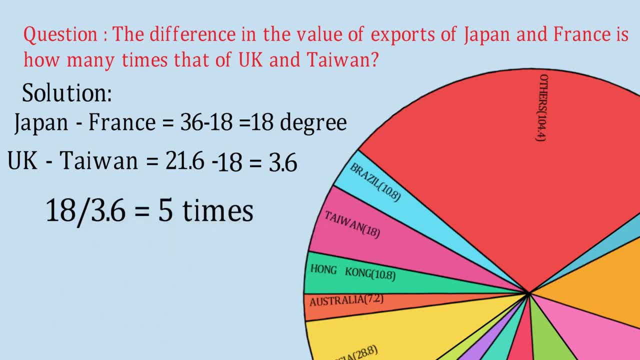 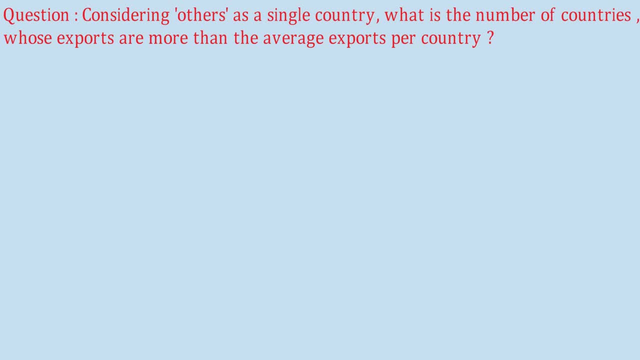 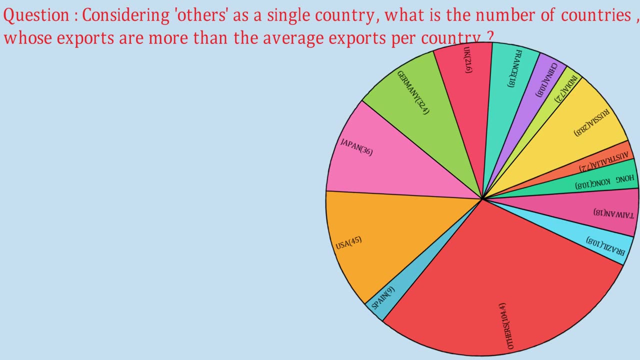 It means that we have to divide the first difference by 5 times. How simple it becomes. Next question: considering others as a single country, What is the number of countries whose exports are more than the average exports per country? There are various countries being depicted in this pie chart. 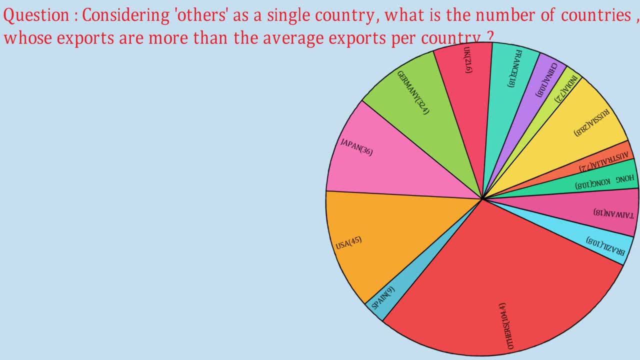 Out of this there is a portion, name as others, which is a large portion, The large red portion, as you can see. So the question says that if you consider others as a single country, So consider it as a country. What is the number of countries whose exports are more than the average exports per country? 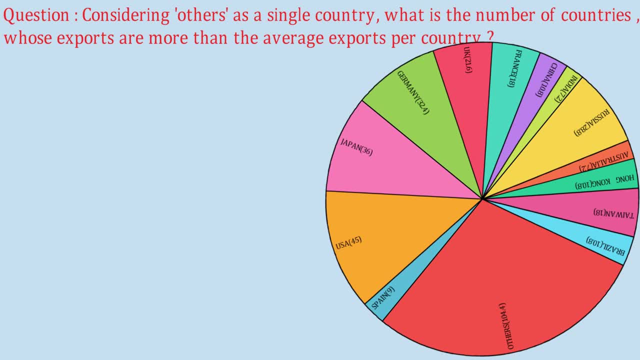 So first of all we have to calculate what is the average export per country. In the question we are given the total exports, That is, the total global export is 72,000 billion dollars And, as we can count, the total countries are 14 in the pie chart. 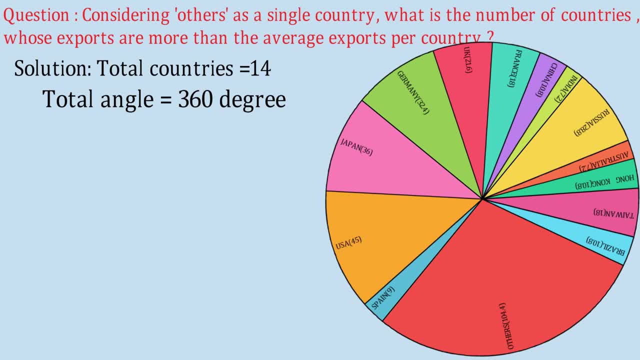 So the total angle being covered by them is 360 degree. So the average angle will come out to be 360 by 14, which is 25.7 degree. Now this is the average angle being covered by a single country. Now we need to calculate the number of countries whose exports are more than the average export per country. 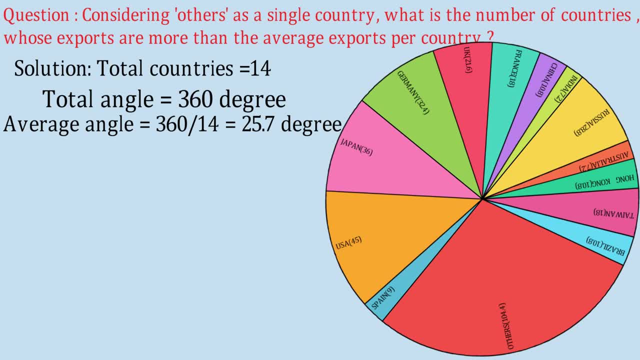 So we have calculated the average export per country, which is 25.7 degree. So let us see what are the individual angles for all the countries: USA, equal to 45 degree. Japan, 36. Germany: 32.4.. UK: 21.6.. 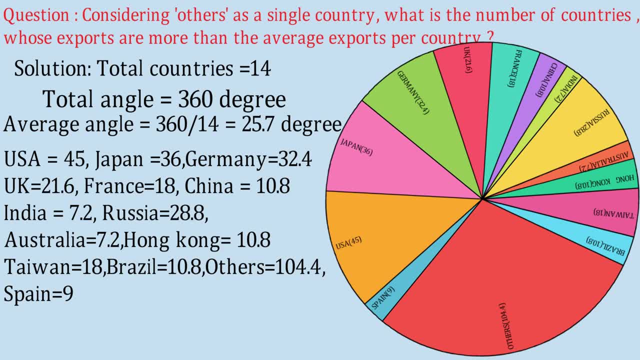 France: 18. China, 10.8. India, 7.2.. Russia 28.8. Australia, 7.2.. Hong Kong: 10.8. Taiwan, 18. Brazil, 10.8.. Others 104.4.. 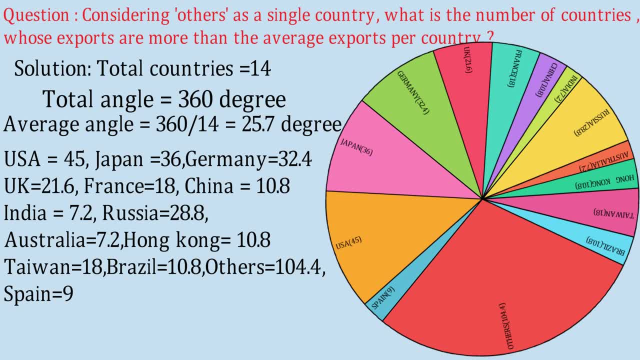 And Spain. 9. Countries who are having angle greater than the average angle, That is, whichever countries are having an angle greater than the average angle, which is 25.7 degree, That will amount for the solution. So USA is having greater angle than 25.7.. 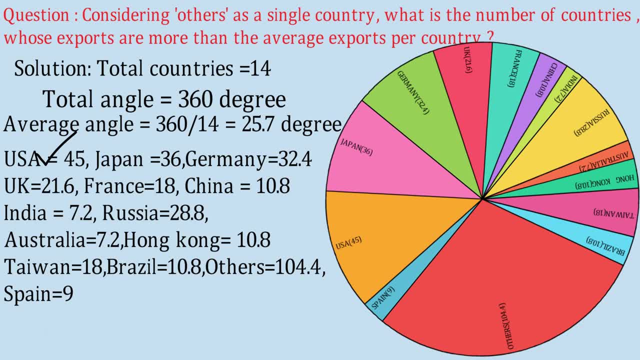 Japan's angle is also greater than 25.7.. Then, as we go next, Germany's angle is also greater than 25.7.. Then we see which is the next country, that is, Russia, is having greater angle than 25.7.. And finally we are having others greater than 25.7.. 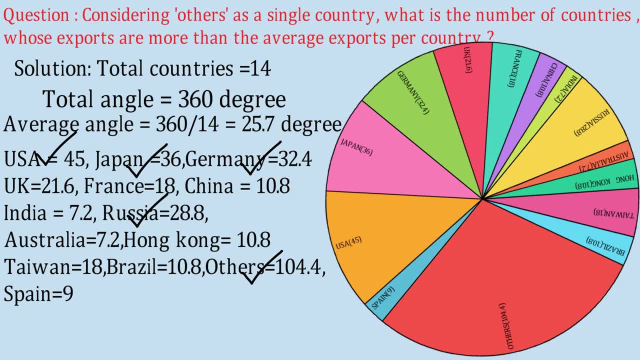 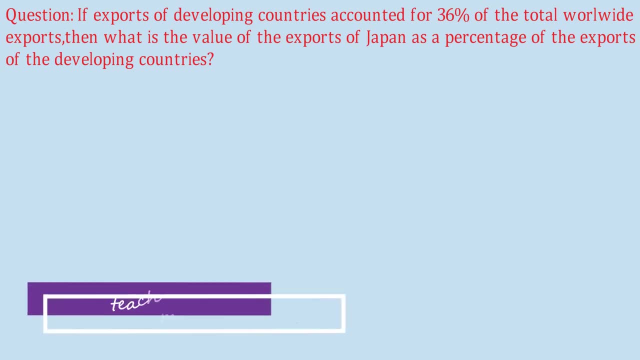 So in all we have 5 countries Having angle greater than the average angle. So that's how simple it becomes when you adopt this methodology of dealing with the angles directly instead of carrying out the wild calculations. Next question: If exports of developing countries accounted for 36% of the total worldwide exports, then what is the value of exports of Japan as a percentage of exports of the developing countries? 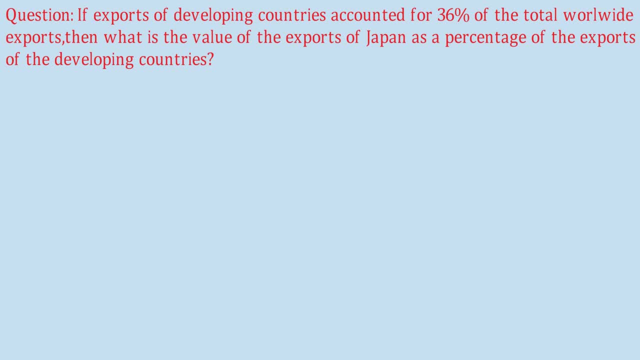 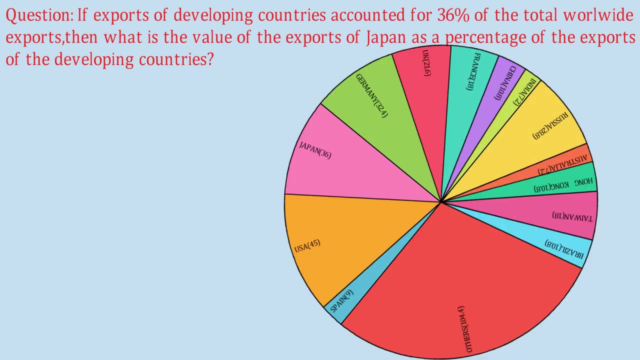 So here we are, being said that the developing countries accounted for 36% of the total worldwide exports And, as you can see, Japan is covering the 36 degree. Total angle covered by the circle is 360 degree, So Japan is 10% of the total. 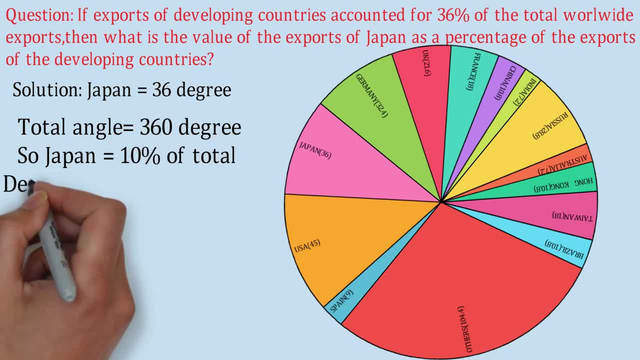 So here we have to compare the percentages covered by countries in this pie chart. Till now we have been dealing with degrees in the pie chart. Now in this question we will deal with percentages in the pie chart. So Japan is 10% of the total. 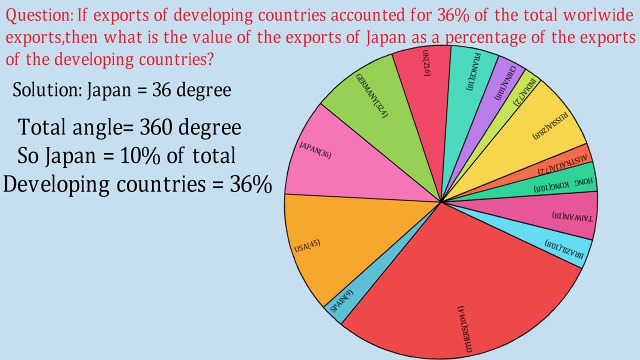 And the developing countries. as indicated in the question, It accounts for 36% of the total, So we can directly compare these percentages. Always remember: we can directly compare these percentages. So as we compare 10 by 36. We get its ratio and when we multiply it by 100. 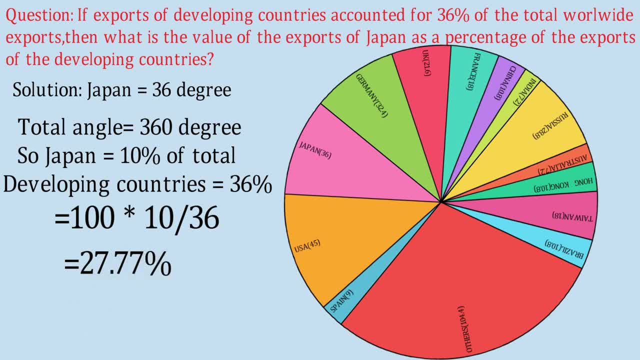 We will get the percentage, because the question says: what is the value of exports of Japan as a percentage of the exports of the developing countries? So we are comparing Japan with the developing countries. The answer comes out to be 27.77%. This is a useful trick.